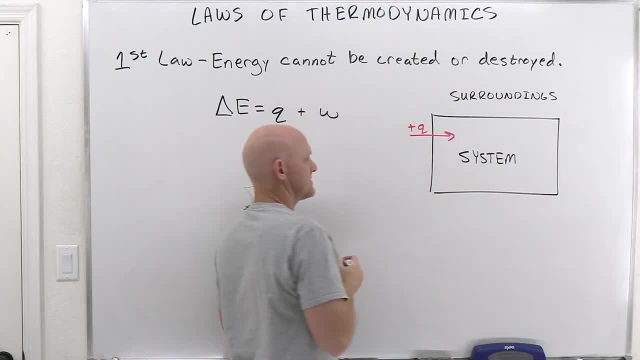 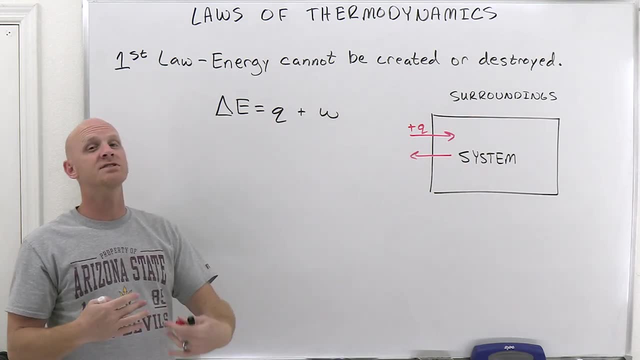 And that is when Q would be positive. So, on the other hand, if heat is transferred out of the system to the surroundings, we always look at it with this equation from the perspective of the system. So in this second example, the system is actually losing the heat, It's losing energy. 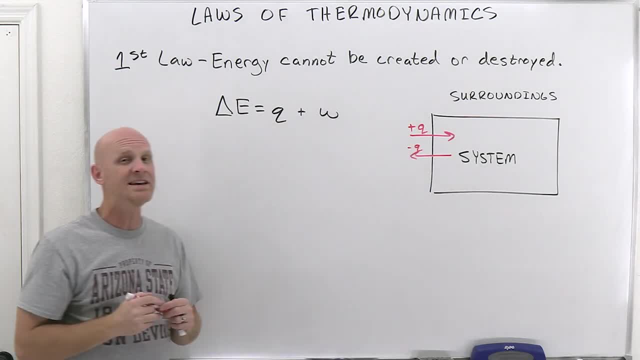 And so that's when we'd have negative Q, That's when Q would be a negative number instead. Now it turns out the other way that energy can be transferred into and out of the system is through mechanical work, And so we've got again same options here, So the system can. 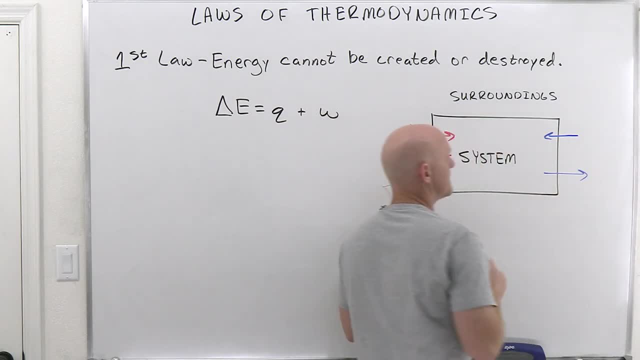 gain energy as a result of work or the system can lose energy as a result of work. And if the system's gaining that energy, we would call that positive work, W would be a positive number, And if the system was losing energy we'd call it negative work. And terminology we learned. 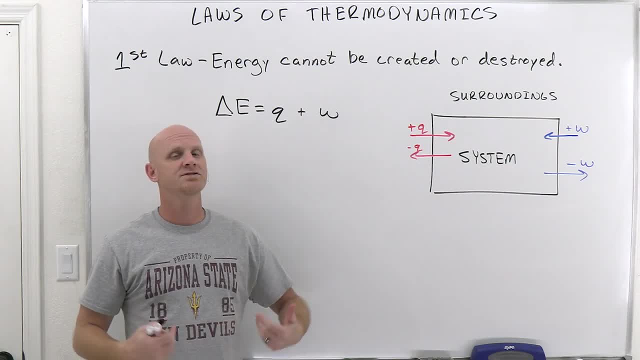 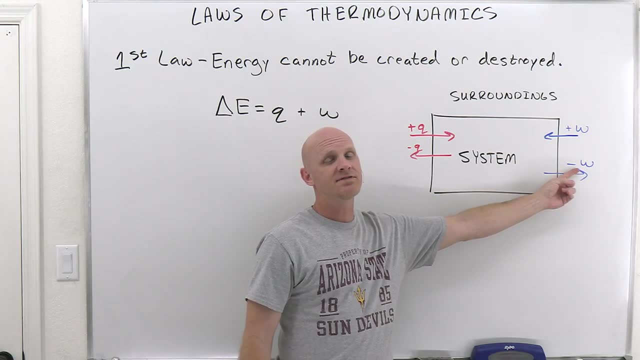 back in chapter five- is that when the system is doing the work, just like if you do work, you're going to use up some of your energy or it'll lose energy. So if the system is doing work, work is going to have a negative value. So- and typically we phrase it- that system is doing work. 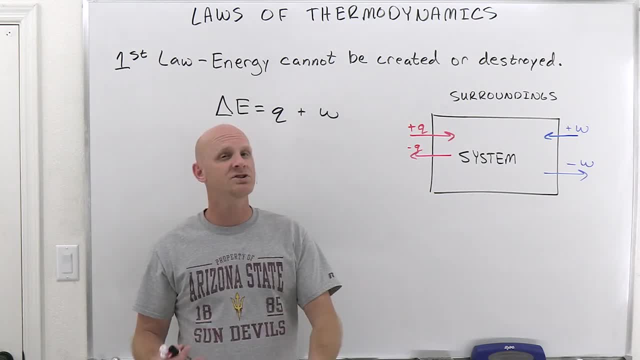 on the surroundings. Now, the other way around, though. if it's the surroundings doing work, well, what are the surroundings doing work on? Well, the only other thing that exists, the system, And so when the surroundings do work on the system, the system is doing work on the surroundings. 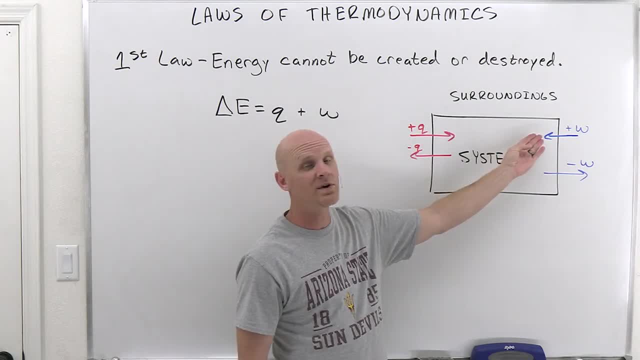 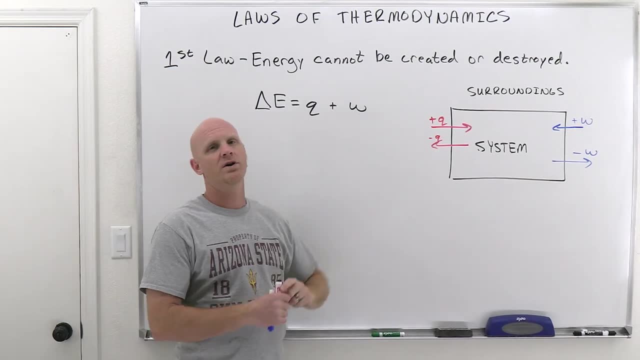 It's now the surroundings that's losing the energy. The system is therefore going to gain the energy, And that would be positive work. Cool Went into a little more detail back in chapter five, And if you want to go back over that, that's totally your prerogative, That's. 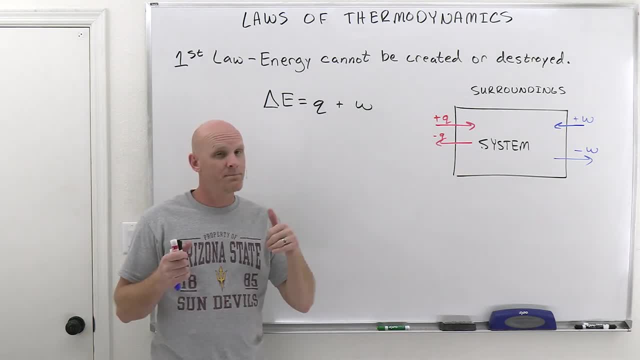 the extent I just wanted to review it here. That's your first law. More important, though, at this stage is going to be the second law of Themenyx. It's new to this chapter and it's the most commonly tested one at this stage of the game, So let's go over that second. 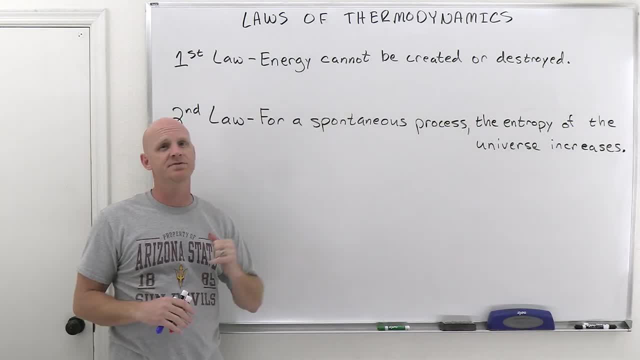 law. All right, So the second law of Themenyx. there are three ways to phrase this That all start out very similar. They all start off saying for a spontaneous process, And spontaneous process is just one that happens without the need for any work being put into. 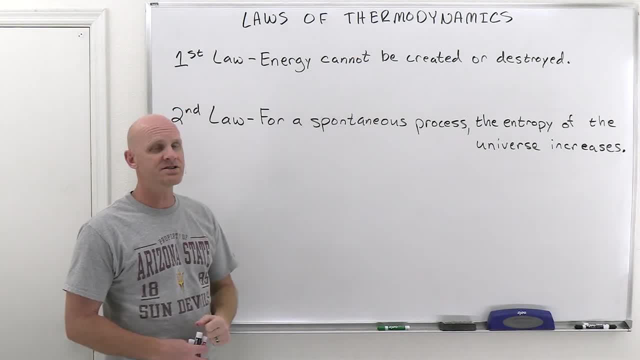 the system. So spontaneous process. we'll get a little better definition of that later in the chapter, but for now it's just a reaction or a process that happens without the need for the input of energy. So you can think of ice melting when it's above zero degrees Celsius. 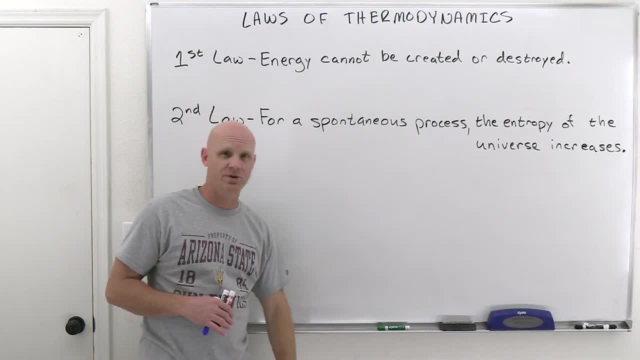 would be spontaneous, whereas ice melting when it's below tell degrees, 0 degrees Celsius would be spontaneous, Whereas ice melting when it's below 0 degrees Celsius would be spontaneous, Whereas ice melting when it's below below zero degrees Celsius would be non-spontaneous things of that sort. So things that happen. 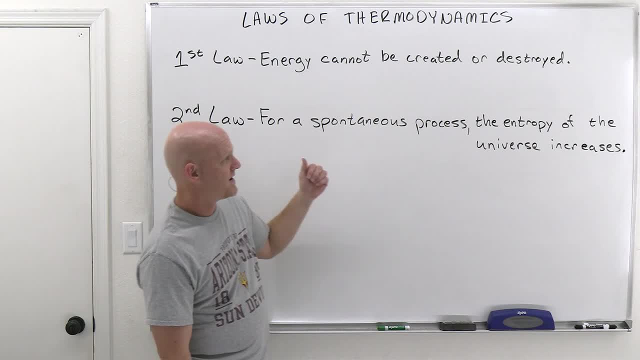 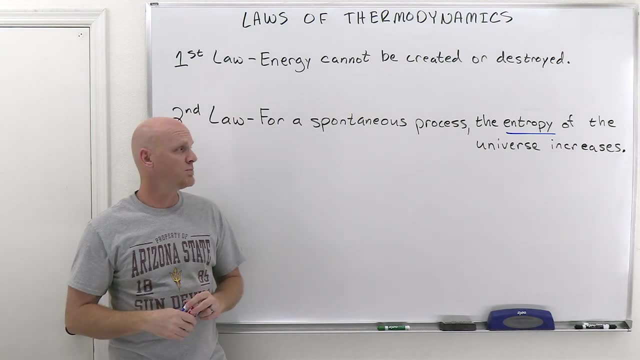 naturally without help, those are spontaneous processes, All right, So where we got to define here those entropy here. So, and that's going to be new to this chapter and that's going to be a big focal point of this chapter. In fact, the entire next lesson is going to be on entropy. 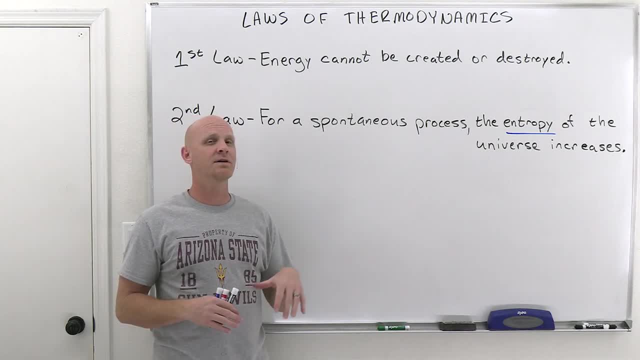 So we'll get more into the nitty gritty of what entropy is in the next lesson, But for now you're just going to want to associate entropy with either randomness or disorder. Now it turns out that entropy is not the same thing, It's not equivalent to randomness or disorder. but you're 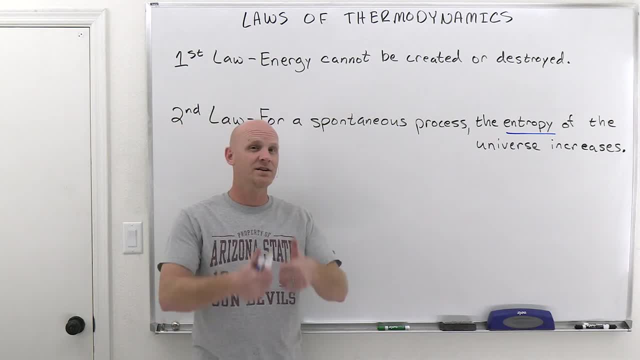 going to want to associate it, because if the randomness or disorder in a system increases, then entropy is going to increase, And if randomness or disorder decreases- ie a system is becoming more ordered- then entropy is going to decrease as well. So they're correlated with. 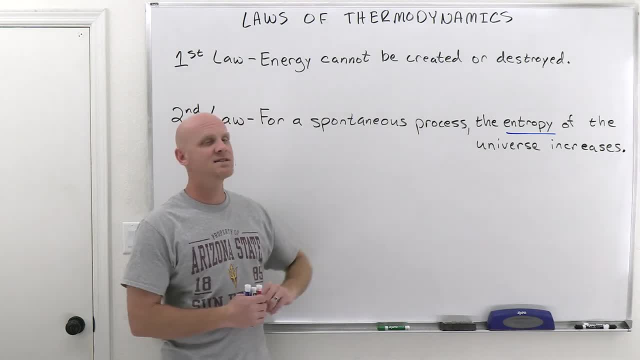 each other, but they're not exactly the same thing. So but suffice it to say, if you can figure out that if a system is getting more disorder, more randomness, then it's going to be getting an increase in entropy as well. 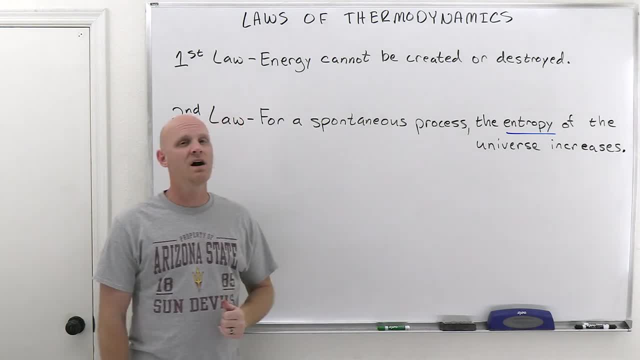 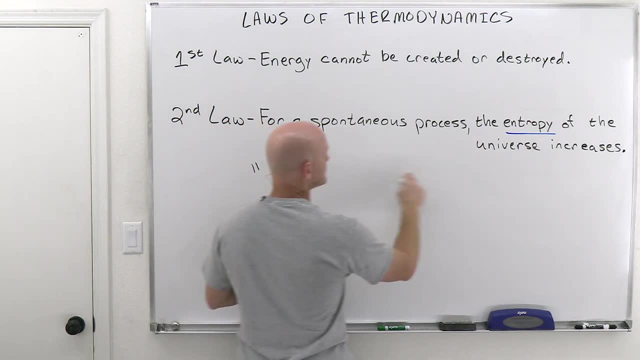 All right, So second law: for a spontaneous process: the entropy of the universe increases. Now there's a couple of different ways. again we can phrase this, And again they're always going to start off with: for a spontaneous process. So, but we can finish this. 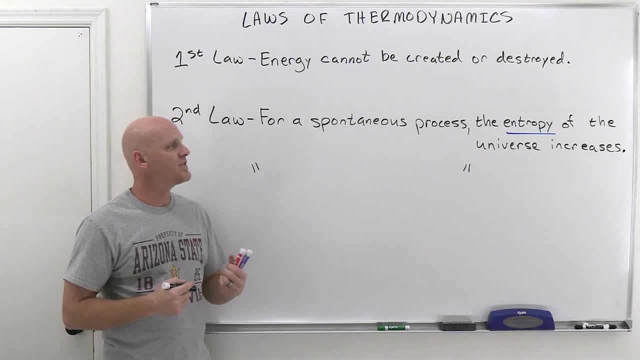 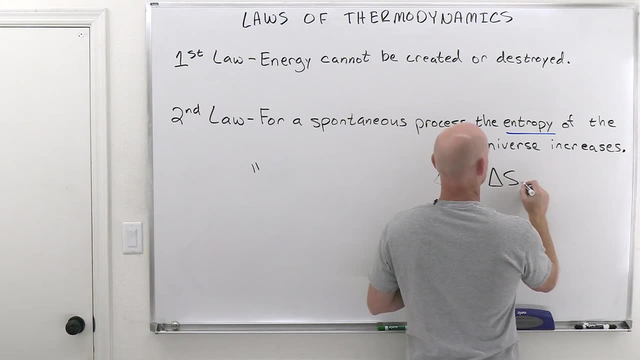 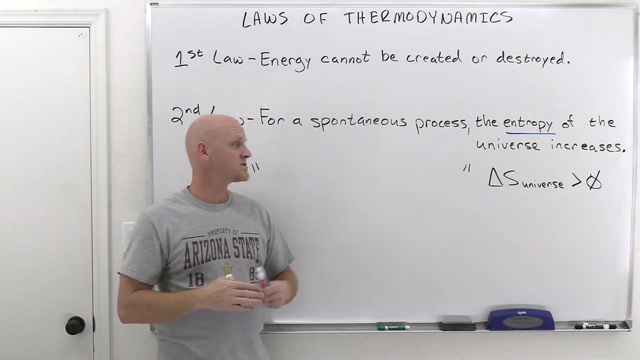 in two other ways that essentially mean the same thing. So so we've got: the entropy of the universe increases. Well, another way to phrase that would be to say, for a spontaneous process, that delta S of the universe is greater than zero. Again, that just means the change in entropy of the universe is a positive 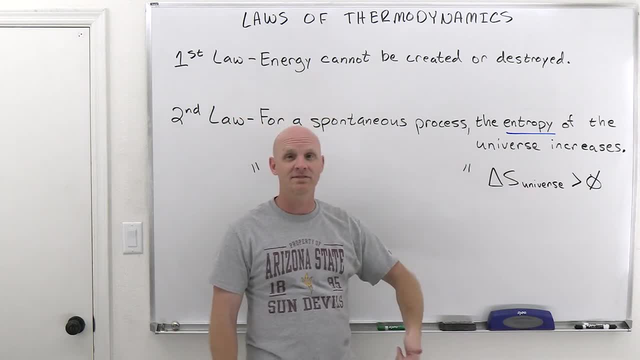 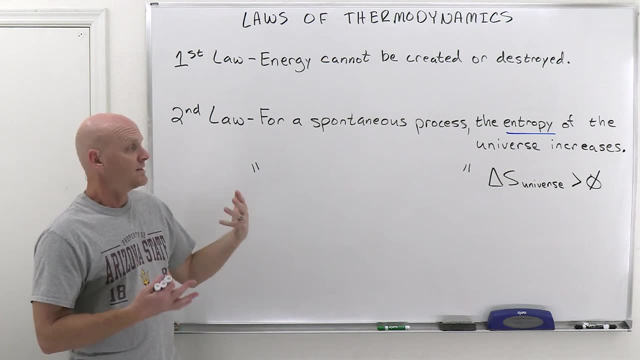 number. Well, it's just if it's, you know, if the change is positive, that means it's increasing, And that's why it means the same thing we said in the first one. So just another way of expressing it. make a little equation out of it. Last one, though, is going to again start off with, for a 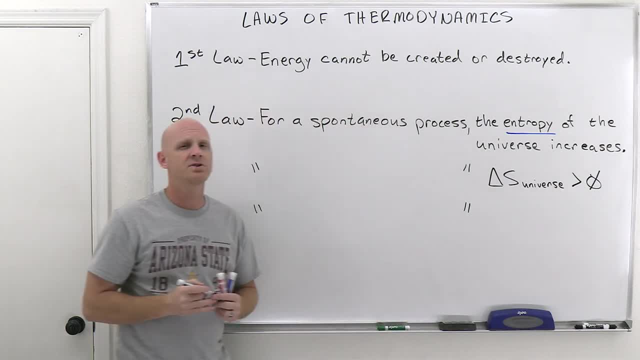 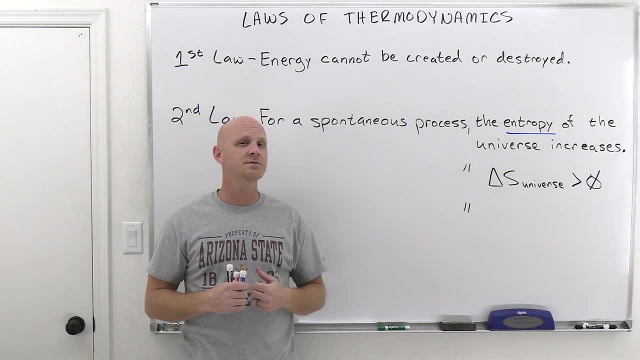 spontaneous process. So, but it breaks up the universe into those two things We said existed when we talked about the first law. there's two things in the universe. there's whatever you're looking at And we call that the system. And then there's 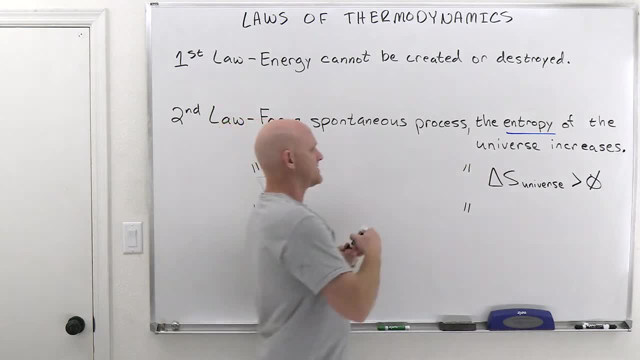 E S everything else in the universe, and we call those the surroundings, And so in this case we could break up that change in entropy of the universe into the system and the surroundings, which I'll abbreviate S-U-R-R and the total between the two. 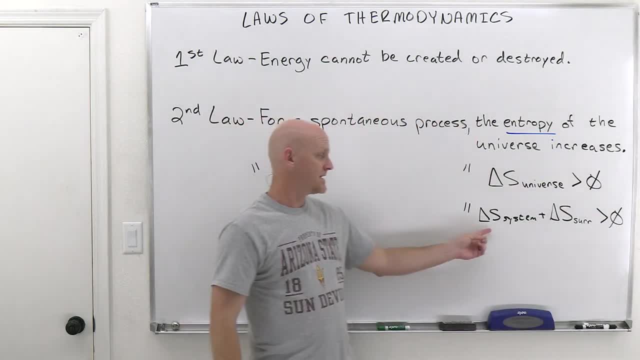 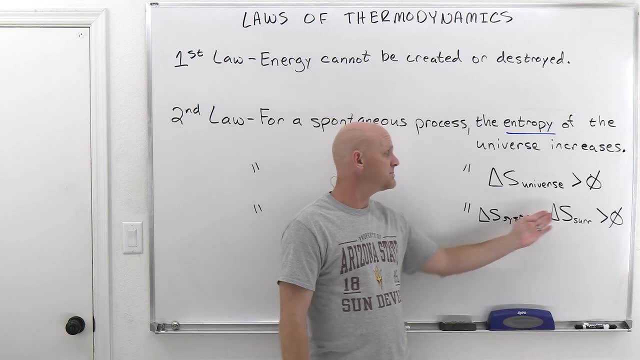 the sum between those two has to be positive And again because the two of them combined are the entire universe. So if the delta S of the universe must be positive for a spontaneous process, well then system plus surroundings must be positive as well. And notice that doesn't mean. 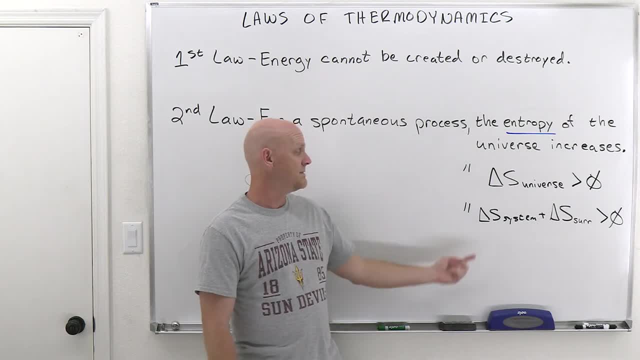 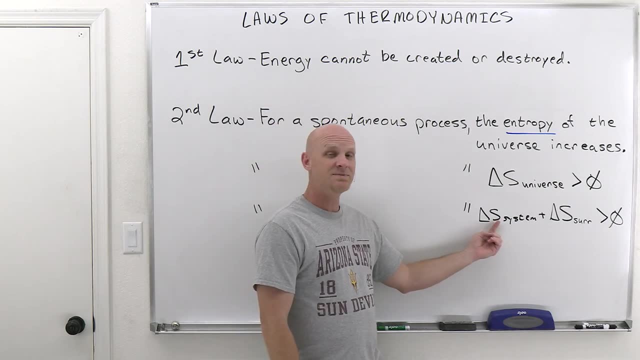 that the delta S of the system has to be positive all by itself, because if the delta S of the system is negative, that's actually okay. That happens all the time. So. but if the delta S of the system is negative, that means that the delta S of the surroundings for that spontaneous process 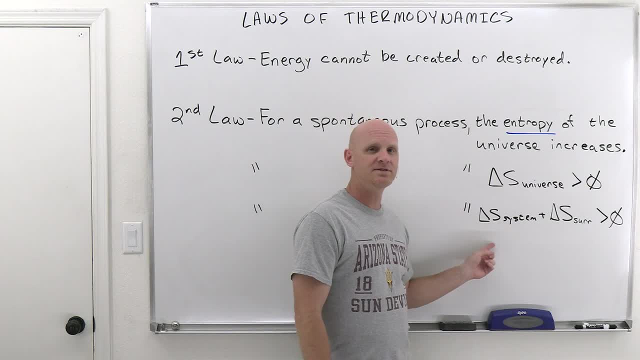 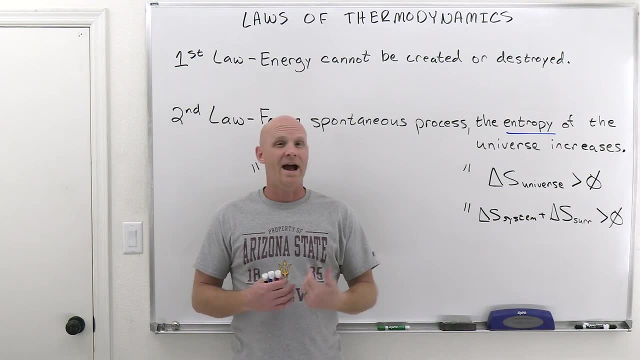 would have to be even more positive. That way, when you add them together, you still get a positive number. So we start looking at this. We'll find out when we talk about the delta S of a reaction In subsequent lessons. when we talk about the delta S of a reaction, we're only looking at just 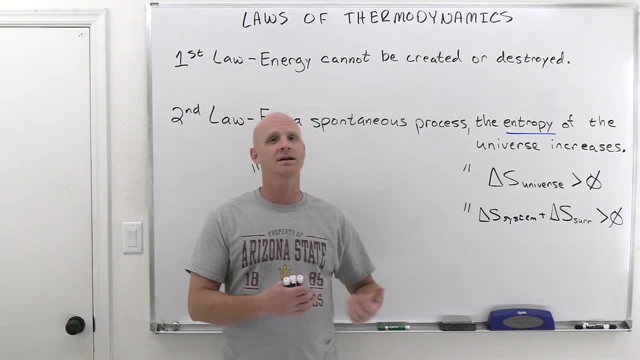 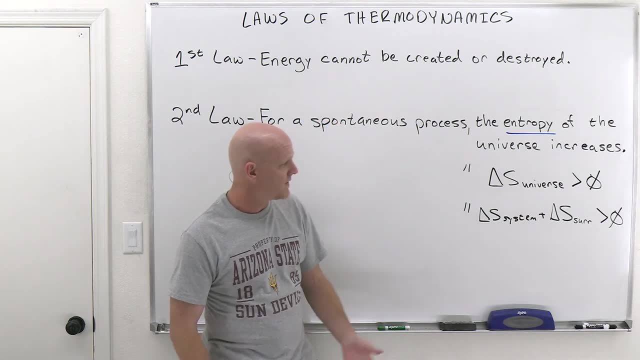 the system And the delta S of a reaction can be positive or negative, And in the next lesson we'll learn how to predict. you know, by looking at a reaction whether it might be positive or negative in many cases, So just keep that in mind: Delta S of a reaction can be negative. 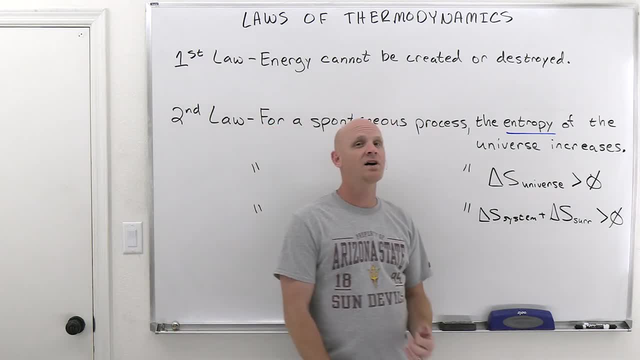 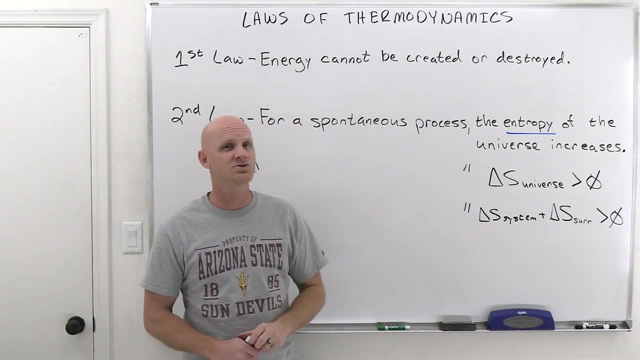 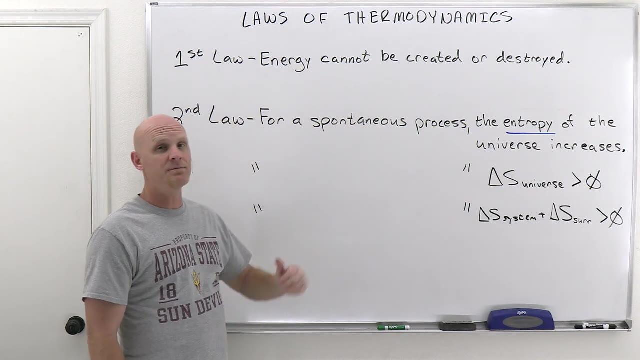 So, however, if you factor in also the surroundings on top of that, for any spontaneous process- again, it always starts off, for any spontaneous process, the delta S of the system plus the delta S of the surroundings. All right, So that's your second law. You're going to want to be able to. you know, just verbatim know. 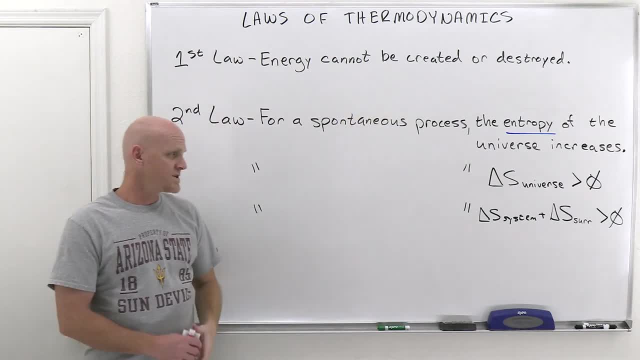 it in any one of these three ways. So all the words, that definition are important, And again, it's the most commonly one you're going to be tested on. So, and then, finally, we've got the third law of thermodynamics. So, and third law talks about a perfect crystal. 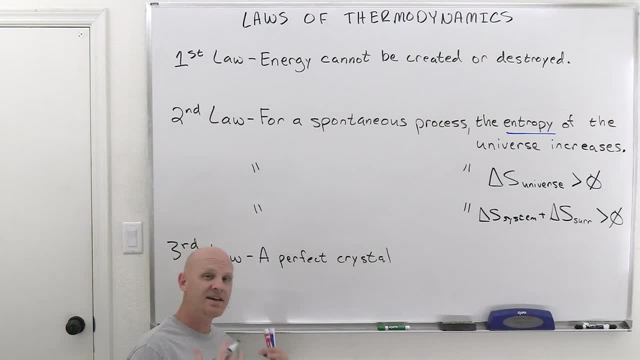 And so a perfect crystal. here we're going to talk about having no impurities. It is a single substance, There's no impurities, So, and it's in a perfect crystalline form, where all the atoms or molecules occupy the exact crystal lattice positions they're supposed to. So a perfect crystal. 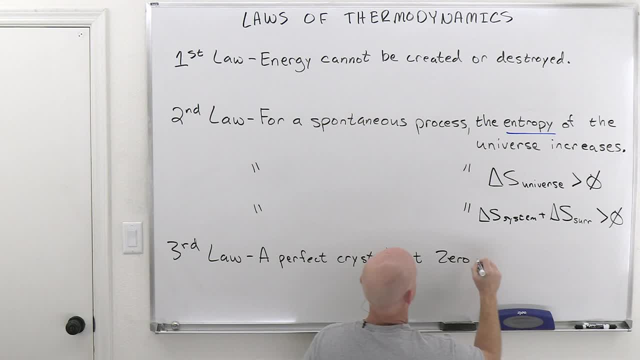 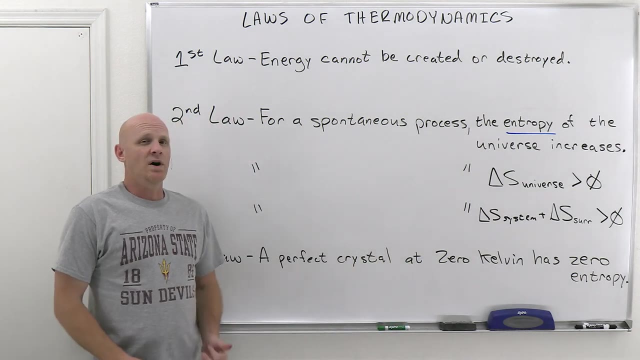 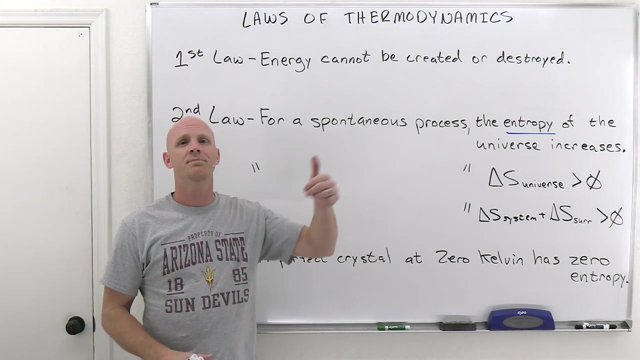 at zero Kelvin has zero entropy. Cool, So you don't want to memorize this as well And a little bit of an understanding you want to get from this. So it turns out that entropy is temperature dependent. As temperature goes up, randomness and disorder go up and so does entropy, And so it turns out as you, cool. 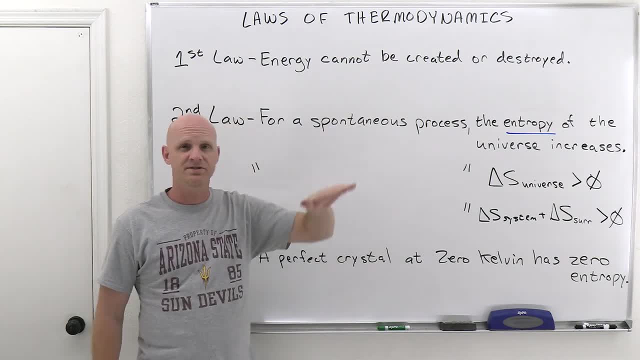 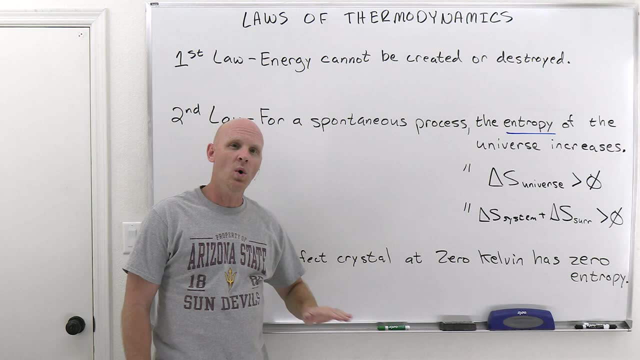 so you know any, pretty much any substance, as you cool them down, their entropy is going to decrease. And as you cool them down it turns out you always hit this minimum point. So and you kind of follow this line back on a curve and stuff like that And you always hit this minimum. 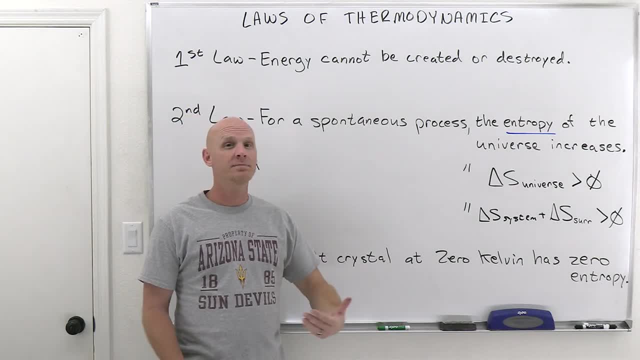 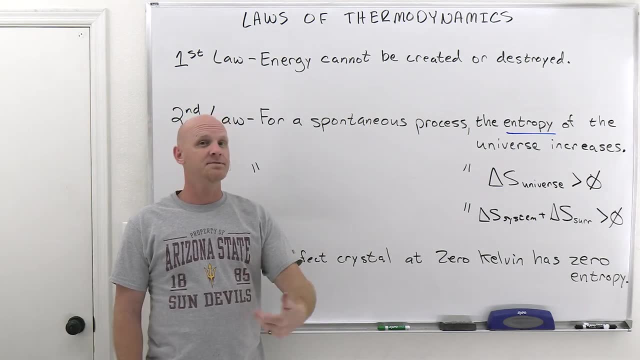 point And you kind of follow this line back on a curve and stuff like that And you always hit this point And they all actually point back to the same minimum theoretical temperature, absolute zero Kelvin, And when they get there, that's the absolute minimum that that substance can have. an. 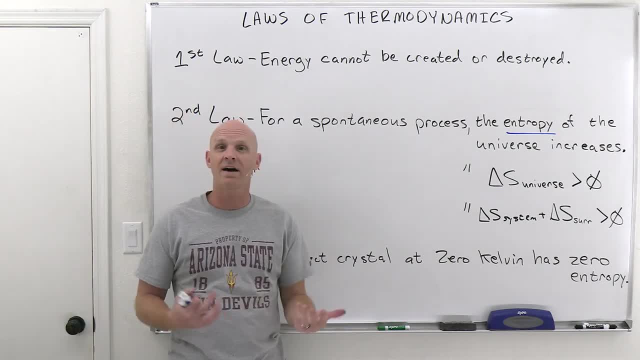 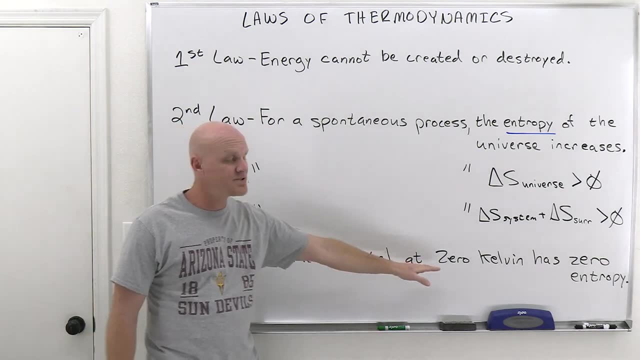 entropy as well, And we give that value. If you can't have a lower entropy than that, well then that's your zero point. So cool, And so it turns out. if you take any perfect crystal and you cool it all the way down to absolute zero on the Kelvin scale, it has no entropy at that point. And we'll. 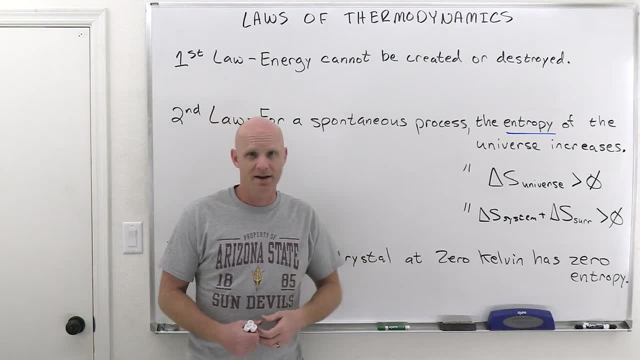 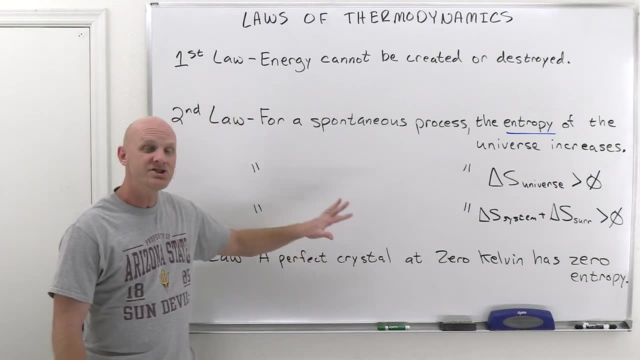 talk about this a little more in the next lesson when we better define it- entropy and go through. you know how we can increase or decrease entropy and how predicted for different reactions. But suffice it to say for now, just memorize this definition. after the next 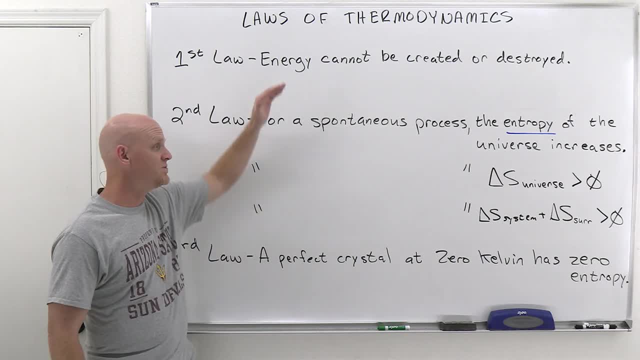 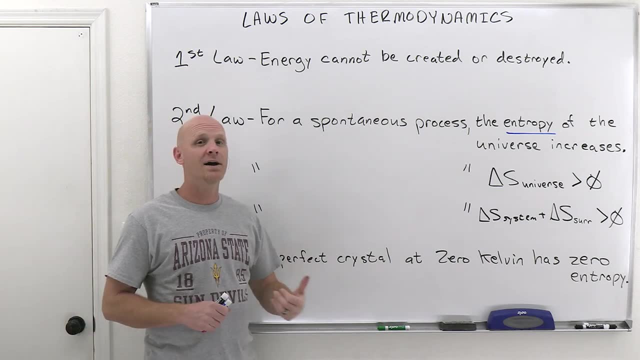 lesson. it'll make a little more sense, But those are your three laws. you need to memorize them And you need to recognize which one is the first and which one is the second and which one is the third law. So you need to recognize them by number- super important. Now, if you found this lesson, 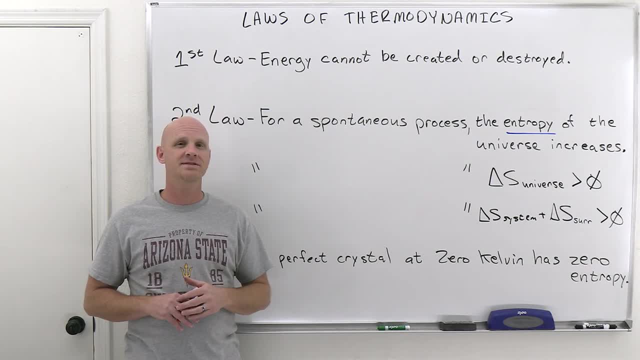 helpful, a like and letting me know in the comments. it's pretty much the best thing you can do to support the channel And if you're looking for more videos like this, please subscribe to the channel. And if you're looking for general chemistry practice materials, study guides.